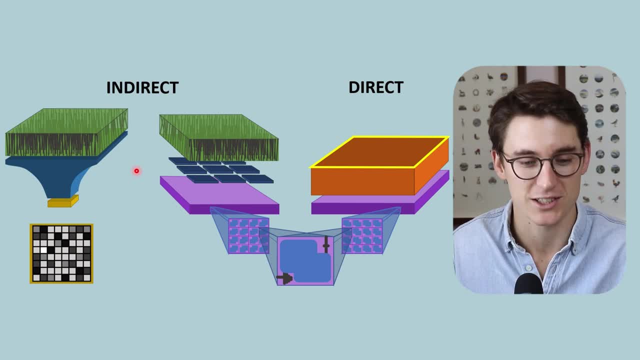 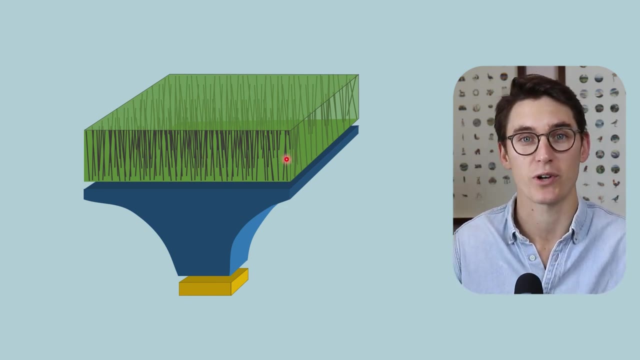 system falls under the indirect digital radiography systems, because x-rays are required to be converted into light prior to an electronic image being created. Now, our CCD system itself has three separate layers. The first is the scintillation layer that we've looked at already: The cesium iodide crystals that 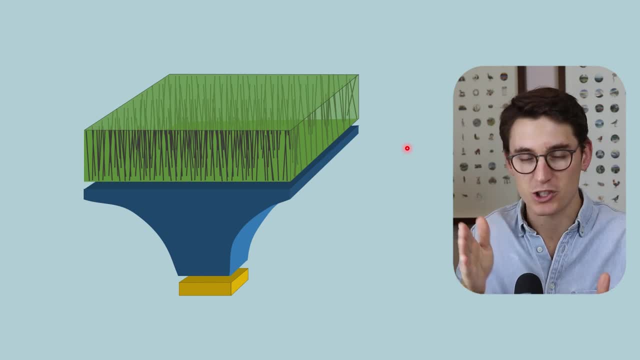 form these long tubular structures that allow light photons to be funneled into a small section in the second layer here. So this scintillation layer takes out X-ray and converts it into light photons. The second layer in a CCD system is known as the coupling layer. The system is called a charged coupled device. This 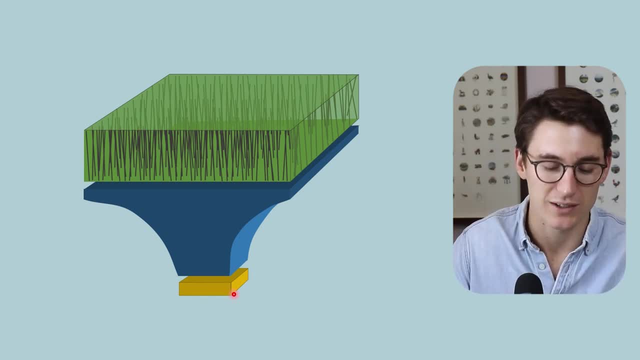 is the coupling layer that couples our light photons to our CCD chip. Now, the coupling layer can be made of two different things. The first of fiber optic coupling. Now, if you're an 80s or 90s baby like me, you would have had 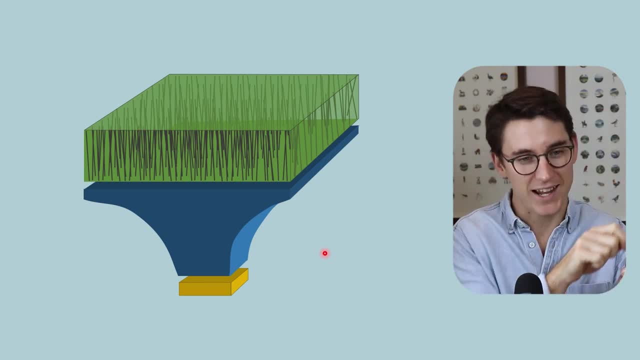 those lamps next to your bed, with those fiber optic lights, and as you move that plastic wire, the light will then be coming out of that plastic wire, which will then be connected to the smells you can hear. Now our CCD system gives us a changes with that fiber optic wire. It's a similar concept here: The light striking this portion of 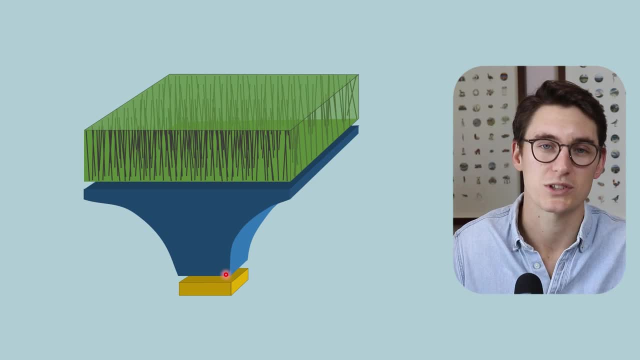 the fiber optic coupling will be funneled down towards our CCD chip. The second type of coupling device is a lens that can focus that light down onto our CCD chip. Now we are taking x-ray photons, converting them to light photons and then converting them into electrons. Now photons. 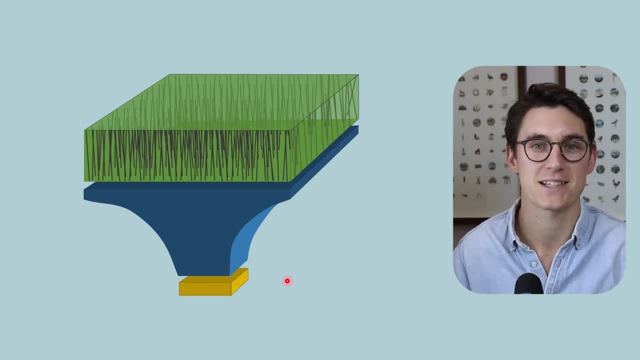 and electrons are both quanta, They are packets of mass and energy And ideally we would like the mass and energy, the x-ray photons here, that energy to equal the electron energy here. We don't want drop-off of that signal, And drop-off of that signal is what's known as secondary quantum sync. 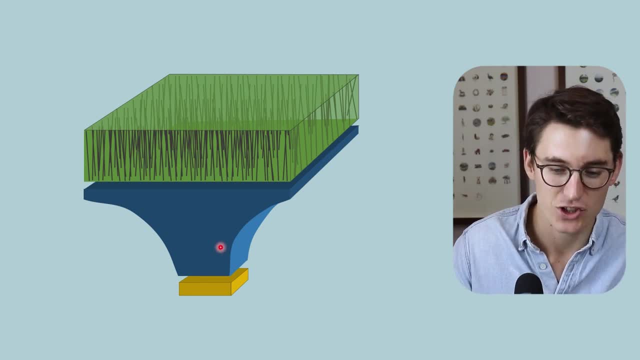 Now that's in fact what we do get here. Our x-ray energies are not the same as those electron energies. here We get drop-off of those energies Because of this coupling that is required. Now, the second reason we get drop-off is because we've got 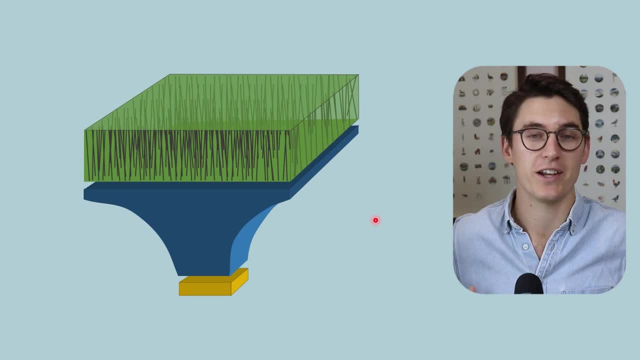 a really large area here. If we're taking an x-ray of a large body region and we need to focus that down onto a very small chip, These chips are small enough to fit in the camera. They are tiny And we are focusing that light down And there's always going to be a loss of some resolution whenever we 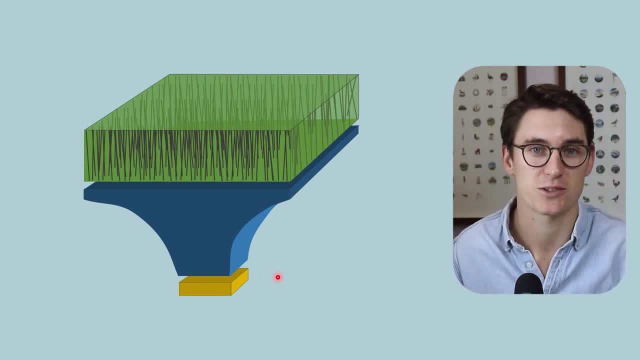 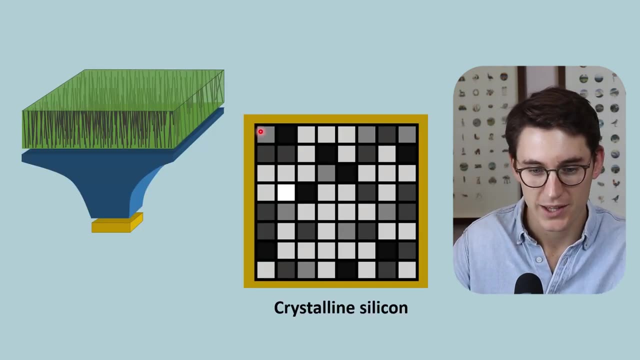 need to take such a large area and focus it down onto such a small area. Now, if we were to flip the x-ray and look at it front on, this is what it would look like. here There will be multiple small functional units on this crystalline silicon face. Now these units here are what are known as dexels. 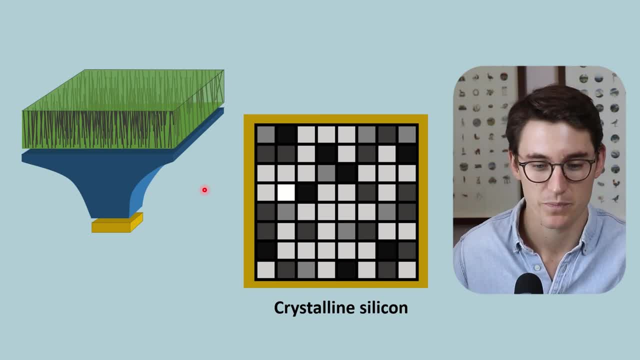 And dexels correspond to the pixels within the image. Now light is being coupled from this scintillation layer to our CTD chip, either by the fiber optic channels or by the lenses that we use, And as that light strikes the silicon layer, electrons are released from the surface. 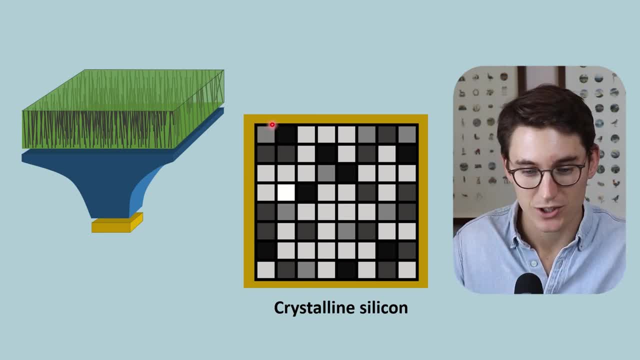 Now the dexels here are separated by voltage gates here that have been etched onto this crystalline silicon. Now the voltage that is run through these black lines here that separate each of these dexels prevent the electrons that have been released on the surface to spread into other. 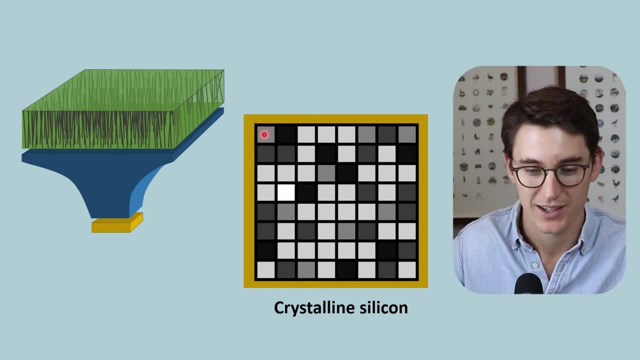 dexels. They keep them within this specific spot. Now, each dexel corresponds to an x-ray intensity that is hitting our scintillation layer. The higher the x-ray intensity here, the more electrons that are released within that dexel. Now, when we want to read out these dexels, we can 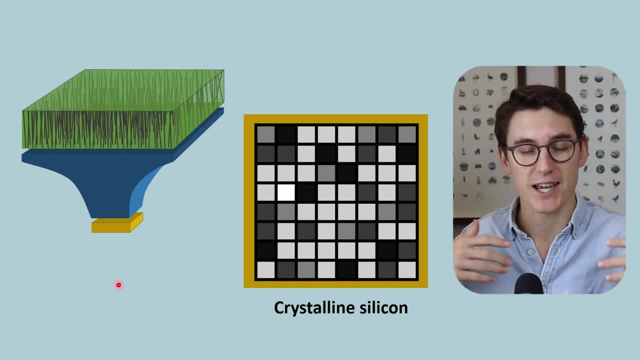 change the voltage along these voltage gates and allow those dexels to be released into what is known as an amplifier, and then that signal can be digitized into a pixel value, a grayscale value that we can represent on our computer screen, ultimately making our radiograph that we've taken. 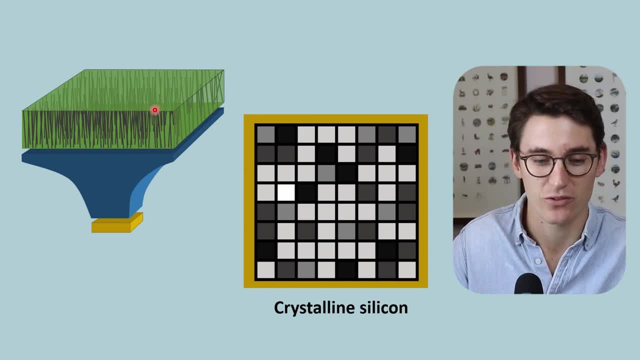 Now the number of electrons again corresponds to the intensity of the x-ray here and as we then read that digital signal, the more electrons that are available, the darker it will appear within that pixel. now the way we read out these ccd chips is row by row. we will allow this entire row to be. 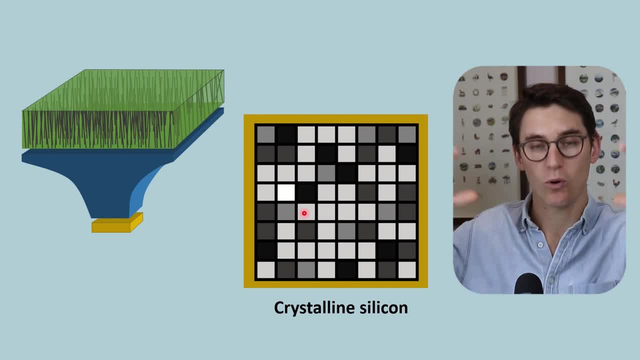 read out, go through the amplifier towards our computer, and then all of these rows will shift down one and we will read out the next one, sequentially, over and over again, and each dexil again corresponding to a particular pixel. so what we've done here is we've taken x-ray energy. 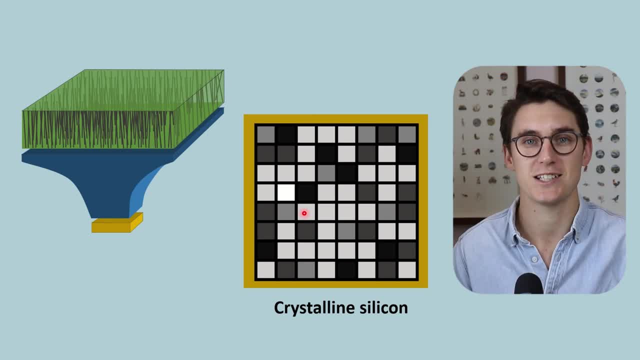 converted it to light, channeled that light down onto our ccd chip. the light hits that crystalline, silicon and electrons are released in proportion to those lights. those electrons are housed within a specific dexil that corresponds to a specific pixel in our image and those dexils are prevented.